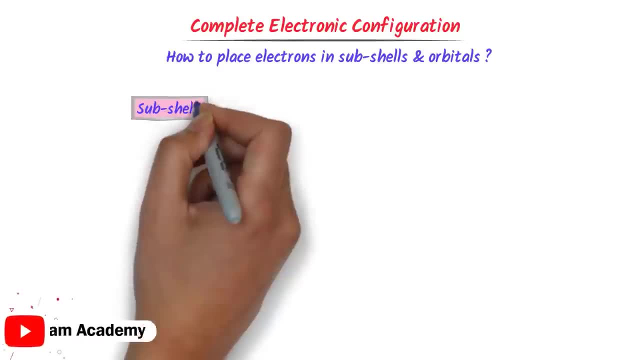 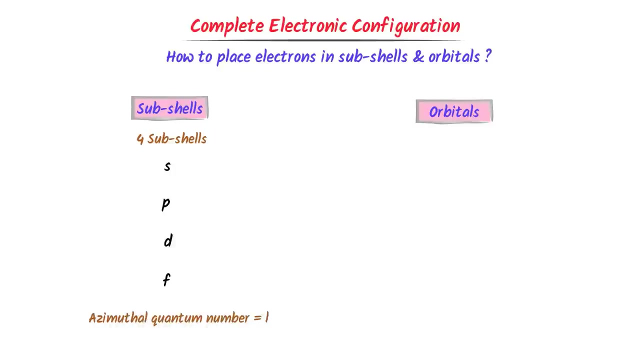 Firstly, let me teach you some key concepts like subshells and orbitals. We know that there are four different subshells, like SPDF, Remember that we represent subshells by azimuthal quantum number, L. For example, when L is equal to zero, it is S subshell. When L is. 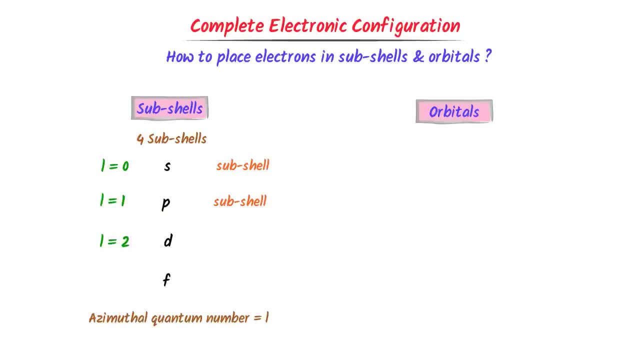 equal to one, it is P subshell. When L is equal to two, it is D subshell. When L is equal to three, it is F subshell. Now, what about the electrons of subshell? Well, I write it. 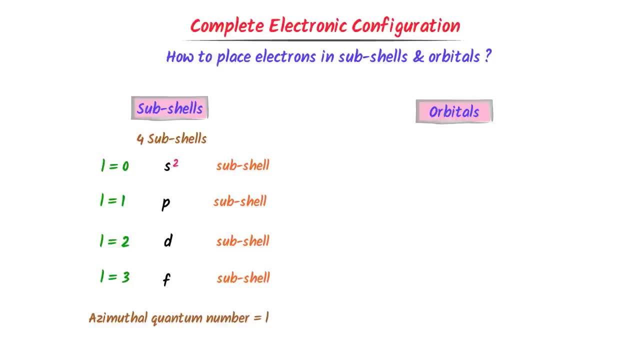 as two electrons, And then I add four electrons successively. Two plus four is equal to six, Six plus four is equal to ten. Ten plus four is equal to fourteen. So S can accommodate two electrons, P can accommodate six electrons, D can accommodate ten electrons And F can accommodate. 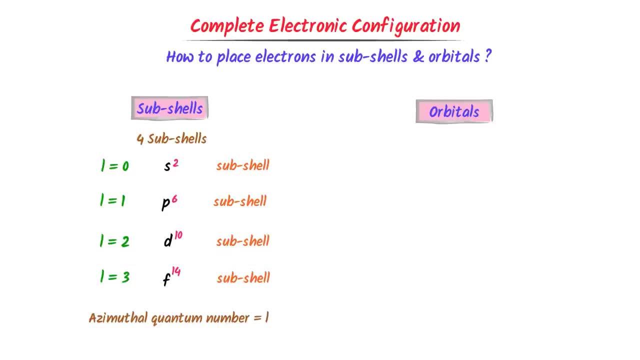 fourteen electrons. On the other hand, every subshell has degenerate orbitals. For example, S subshell has one degenerate orbital, P subshell has three degenerate orbitals, D subshell has five degenerate orbitals And F subshell has seven degenerate orbitals. 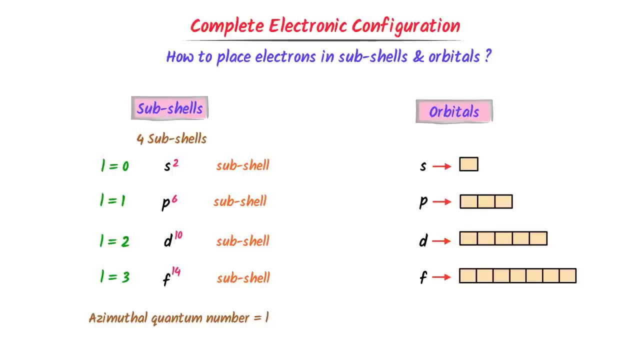 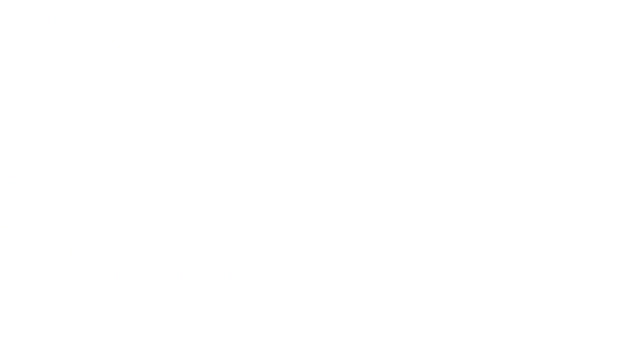 The simple trick is to divide the number of electrons of subshell by two And you will get the number of orbitals. For example, dividing two electrons by two, we get one orbital. Six electrons by two orbitals- 10 electrons by 2, we get 5 orbitals. 14 electrons by 2, we get 7 orbitals. Now, 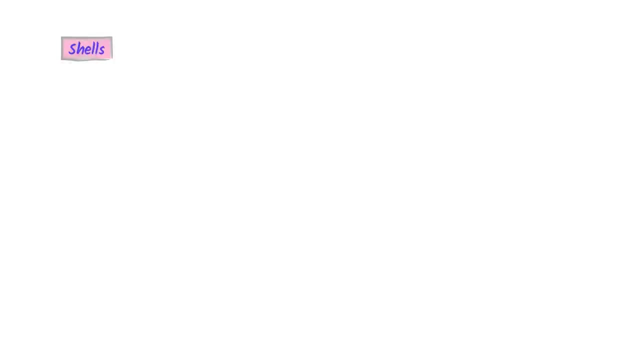 what about the man shells of atom? We know that man shells are represented by principal quantum number. For example, when n is equal to 1, it is K shell. When n is equal to 2, it is L shell. When n is equal to 3, it is M shell. When n is equal to 4, it is N shell. 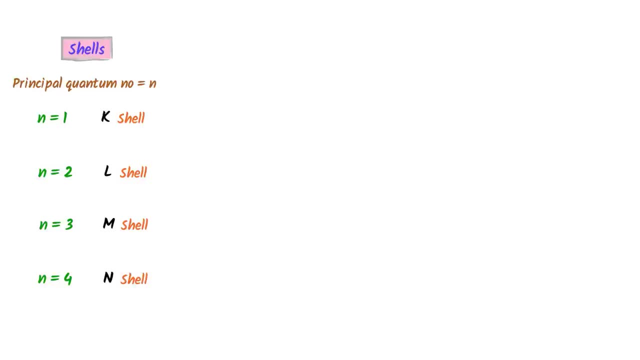 Secondly, we know that every shell has sub-shells. Now how can we learn the sub-shells of man shells? Well, it teach this trick. I write here S and I add one sub-shell successively, like S, sp, then spd, then spdf. 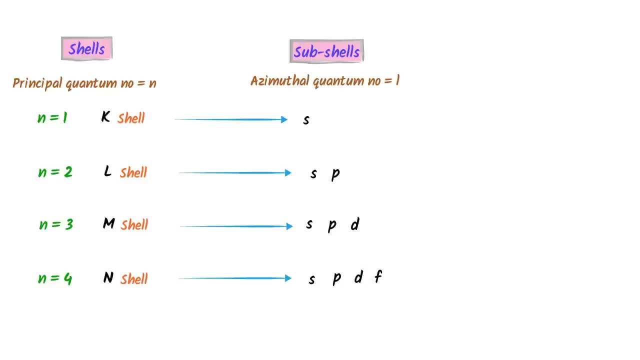 This is s-sub-shell. shell belongs to first shell. I write here: 1.. These are SP sub-shells. They belong to second shell. I write here 2 and 2.. These SPDF sub-shells belong to third shell. I write: 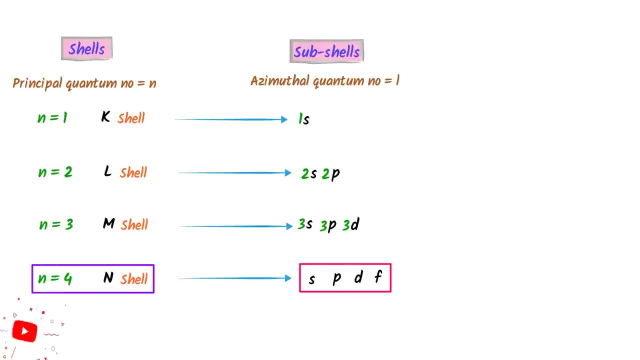 here 3,, 3 and 3.. These SPDF shells belong to fourth shell. I write here 4,, 4,, 4 and 4.. Remember that this 1S is different from 2S. This 1S means it is the sub-shell of first. 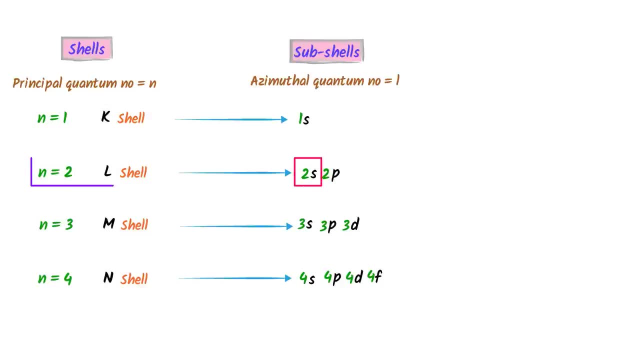 main shell And this 2S means it is the sub-shell of second shell. So remember that 1234 with SPDF represents the main shells. Let me repeat it: These numbers, 1234 with SPDF sub-shells represents the main shells. 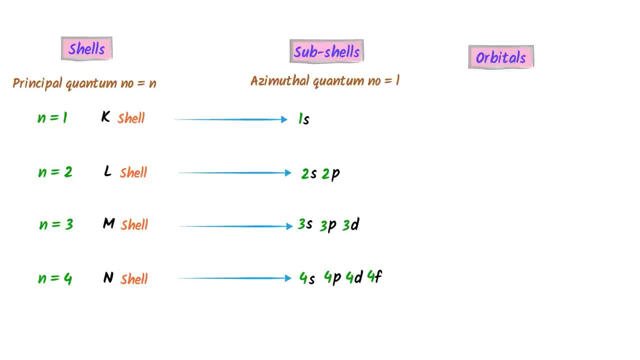 1. Now, what about their orbitals? Well, this 1s has 1 orbital. this 2s has 1 orbital. this 2p has 3 orbitals. Similarly, this 3s has 1 orbital. 3d has 5 orbitals. this 4s has. 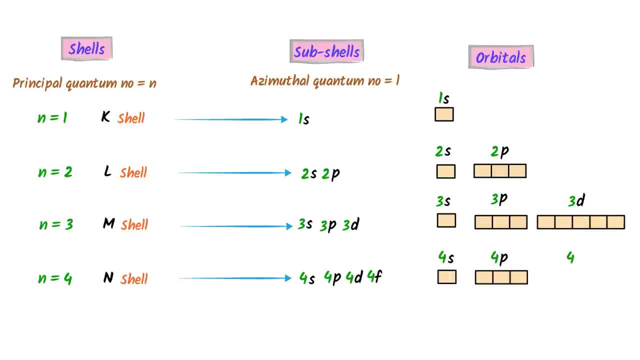 1 orbital, this 4p has 3 orbitals, this 4d has 5 orbitals and this 4f has 7 orbitals. Just note it down, this complete concept of shells, subshells and orbitals. 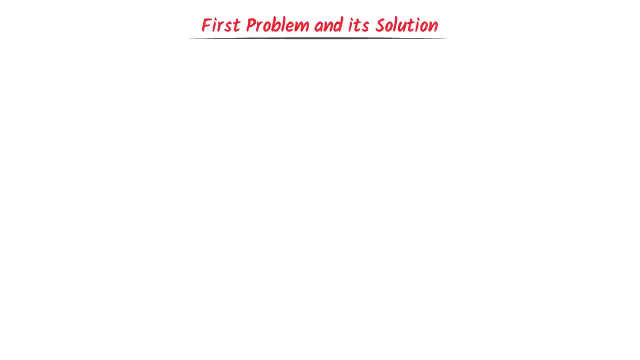 Now we will discuss the first problem and its solution. I mean, how can we place electrons in the subshells? Well, consider a nitrogen atom. We know that its atomic number is 7.. Now the problem is: how can we accommodate the 7 electrons in subshells? Here comes the 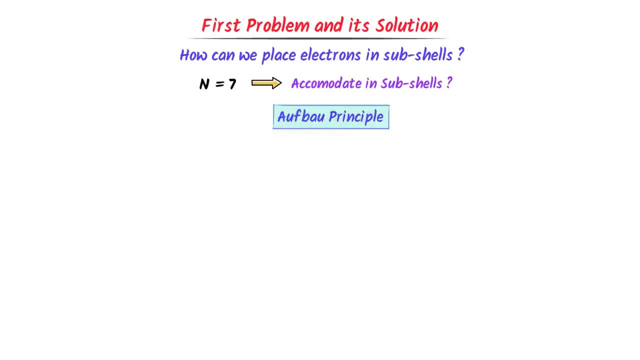 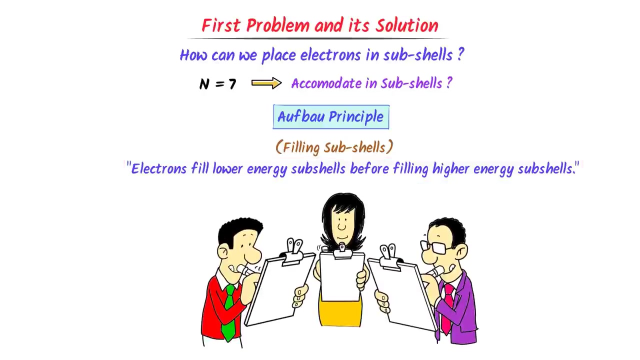 Aufbau principle. Aufbau principle teaches us about filling subshells. Aufbau principle states that electrons fill lower energy subshells before filling higher energy subshells. Let me repeat it: Electrons fill lower energy subshells before filling higher energy subshells. Now here, students do a lot of mistakes and 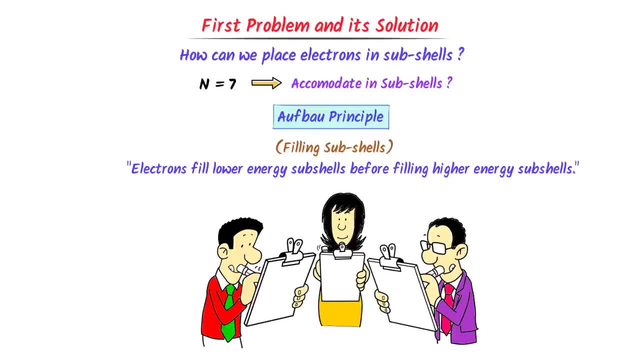 they face big problems. I mean, they cannot remember the order of subshells from lower to higher energy levels. So to solve this problem I teach this easy trick: I write spdf and I write 1234.. I go from back side. I write here s, two times s and s. Then I go from p to s, I write here: 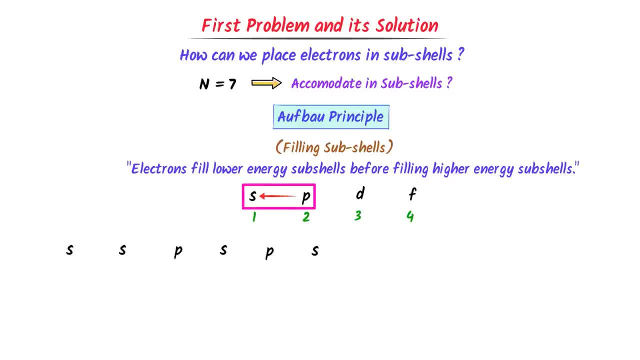 two times ps and ps. Then I go from d to p to s, I write them two times: dps and dps. Lastly, I go from f to p to d to s, I write them two times: fdps and fdps. 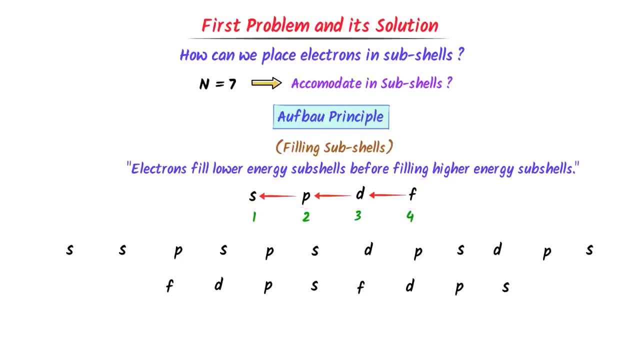 We know that s is the first subshell. I will start numbering the s subshell from 1, like 1s, 2s, 3s, 4s, 5s, 7s, 8s, 9s, 10s, 11s, 11s, 12s, 12s. I get this pdps. I am going to type. fdps, dps, dps, 9s and we will write it twice. So dps and dps. There, dps and dps. we know that I write dps and dps. We know that S is the first subshell. I will start numbering the s subshell. 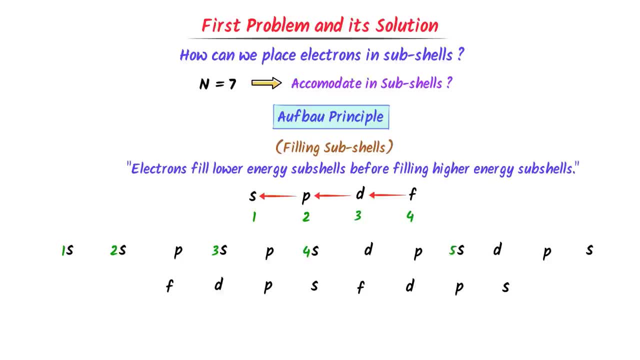 3s, 4s, 5s, 6s, 7s and 8s. Secondly, the p is the second subshell. I will start numbering the p subshell from 2, like 2p, 3p, 4p, 5p, 6p and 7p. Thirdly, the d is the third subshell. I will start numbering the d subshell from 3, like 3d, 4d, 5d and 6d. Lastly, the f is the fourth subshell. The f subshells by 4, like 4f and 5f. This is the order of increasing subshell. 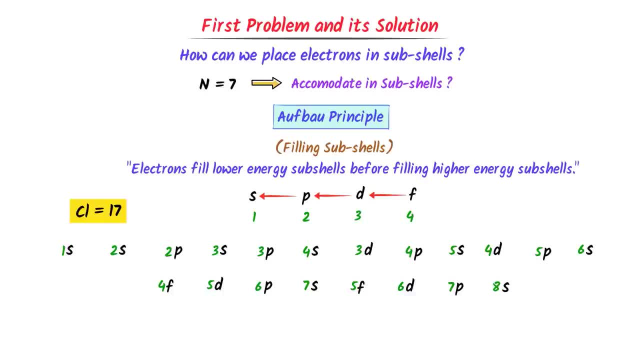 Now consider chlorine atom, and its atomic number is 17.. We already learned that s can accommodate 2 electrons, p can accommodate 6 electrons, d can accommodate 10 electrons, f can accommodate 14 electrons. In case of chlorine, 2 electrons are placed in 1s. 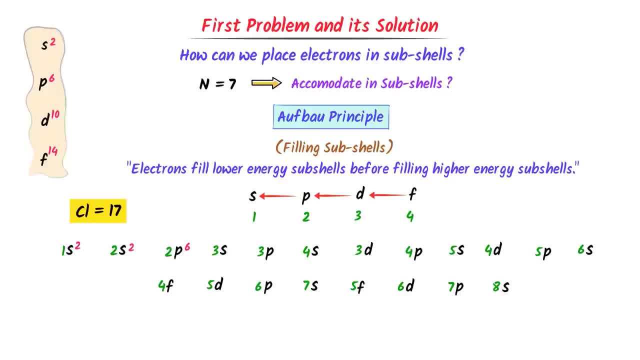 2 electrons in 2s, 6 electrons in 2p, 2 electrons in 3s and 5 electrons in 3p. This is the complete electronic configuration of chlorine and subshells. Thus we learn that Ofbu principle teaches us about filling subshells with the electrons and we use this easy trick. 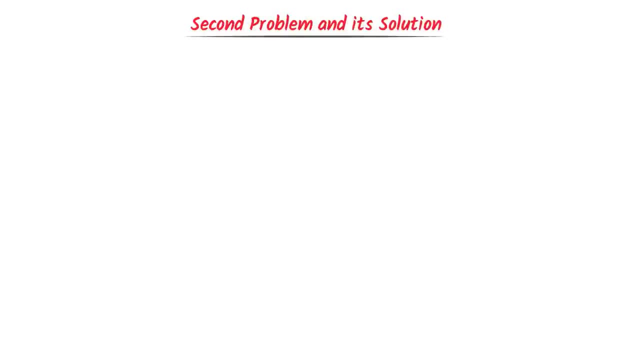 Now we will discuss the 2nd problem. I mean, how can we place electrons in orbitals? Well, to solve this problem we use the Hund's rule and Pauli-exclusion principle. Pauli-exclusion principle states that each orbital of a subshell can accommodate 2 electrons with. 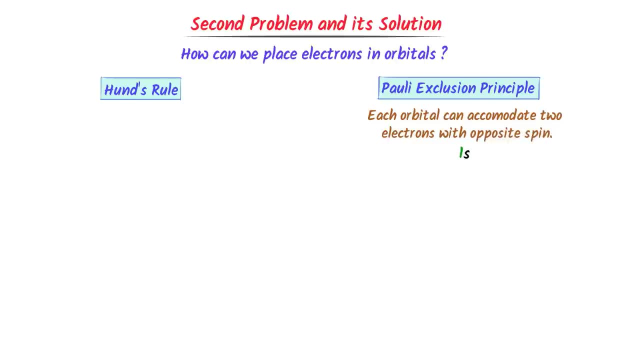 opposite spin. For example, consider this one as orbital. It will accommodate 2 electrons, but the spin of electron must be equal to or equal to 1. opposite. Secondly, Hans rule is all about filling orbitals of subshells. I always teach: 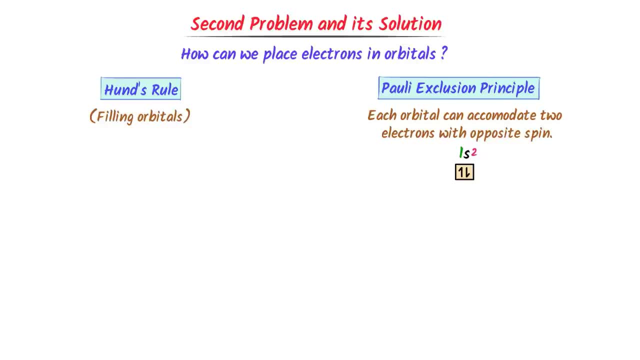 these two important points about Hans rule. Firstly, it states that every orbital is singly filled. before any orbital is doubly filled. For example, consider this 2p orbital. I am interested to place six electrons in it. Firstly, I singly fill it. One electron, one electron. 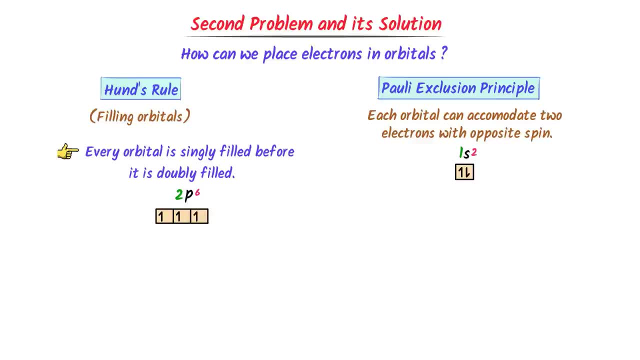 one electron, Then I doubly fill it: One electron, one electron and one electron. So I successfully placed six electrons and two orbitals. Secondly, it states that all electrons and singly filled orbitals have the same spin. For example, consider 2p. 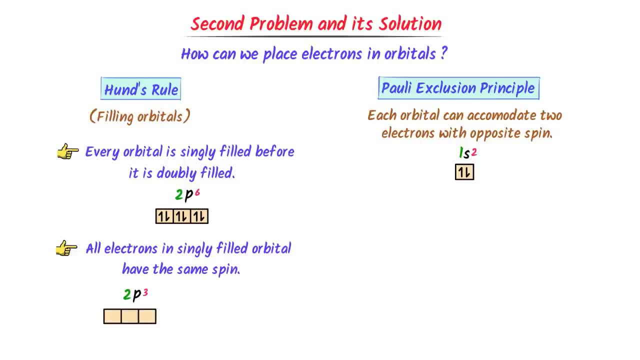 I am interested to place three electrons in it. I place first electron in upward direction, the second electron in upward direction and the third electron in upward direction. Or we can place these three electrons in downward direction. So here all the singly filled orbitals have the same spin. So these both cases are correct. Now we will discuss some. 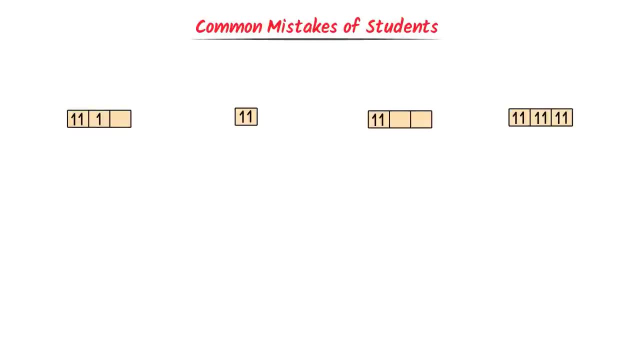 common mistakes of students like these. This is wrong Because, according to Hans rule, firstly we have to singly fill it. I write one electron, second electron and third electron in upward direction, are first electron, second electron and third electron in downward direction. These both cases are correct. Secondly, it 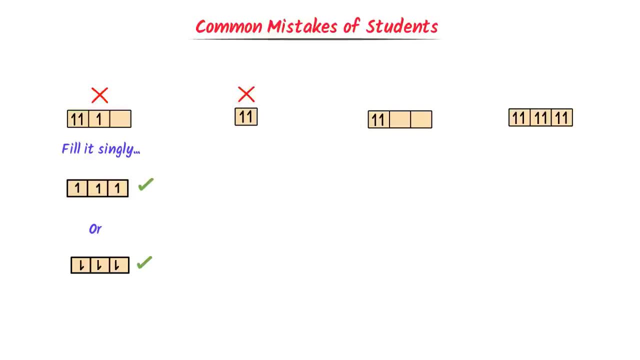 is wrong Because, according to Pauli exclusion principle, their spin must be opposite. So I need to correct the spin: First electron in upward direction and second electron in downward direction. This is correct. Thirdly, it is wrong Because, according to Hans rule, 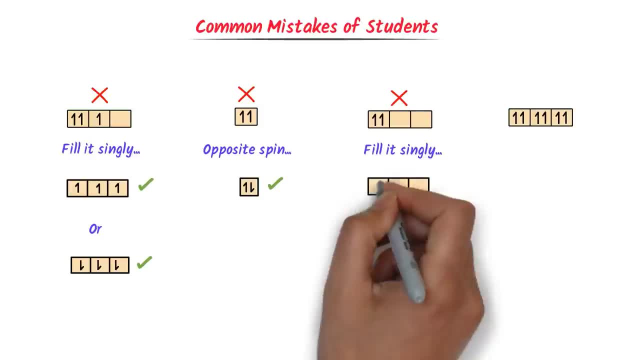 we have to singly fill it Like first electron and second electron in upward direction. Finally, this is also wrong Because these all electrons have the same spin. I write first electron, second electron, third electron and upward direction. Then first electron, second electron. 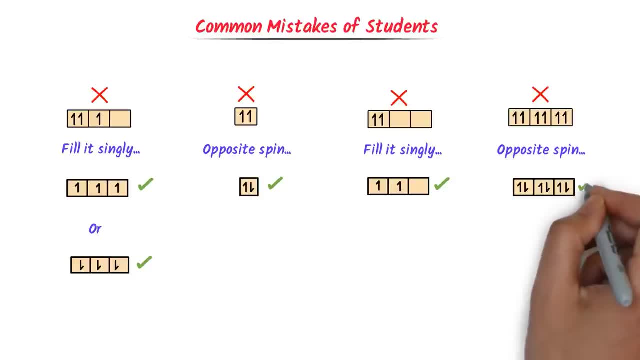 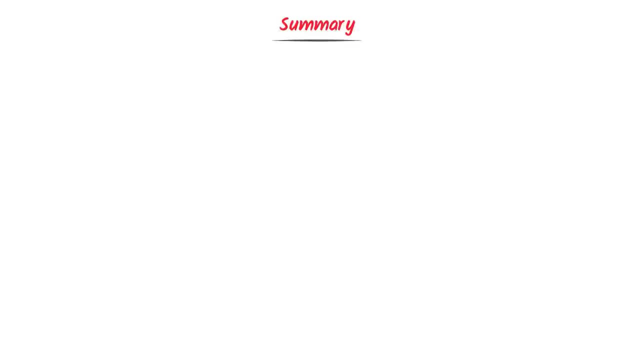 and third electron in downward direction. Now it is correct. The noted down, these common mistakes are the students. Finally, to summarize this whole lecture, let me ask you Configure the electrons of oxygen and subshells and orbitals. Pause the video and try to solve it. Well, I write spdf. 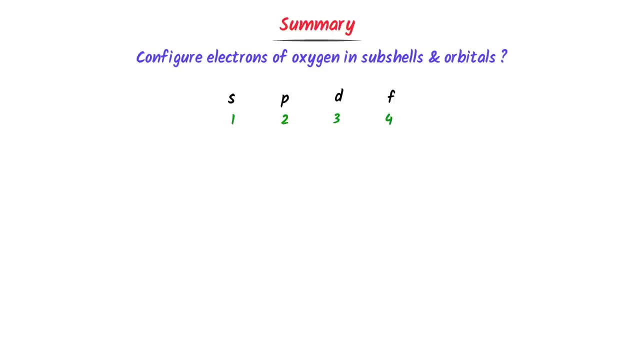 and 123.. go from back side. I write here S two times S and S. Then I go from P to S. I write here two times P, S and P S. I start numbering S. subshell 1,, 2,, 3, 4.. I start numbering. 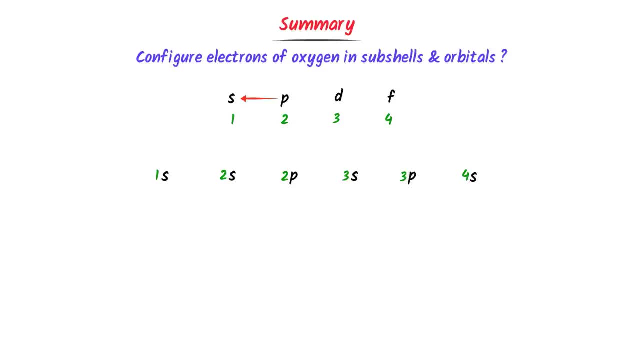 P, subshell 2 and 3.. We know that oxygen has 8 electrons. I place two electrons in 1 S, Two electrons in 2 S, Six electrons in 2 P. Secondly, 1 S has one orbital, 2 S has also. 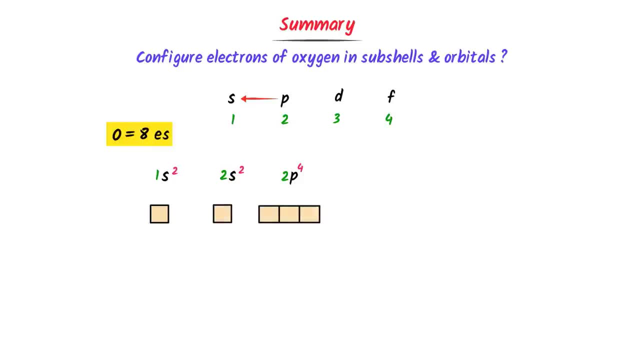 one orbital And 2 P. has three orbitals And 1 S- first electron in upward direction, second electron in downward direction And 2 S- first electron in upward direction, second electron in downward direction And 2 P. I write first electron, second electron and third electron.